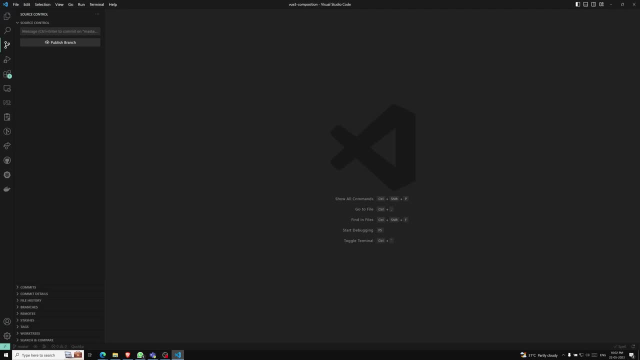 Hi friends, this is Leela. Welcome to my channel, LeelaWebDev. In this video we will see about the custom directives, How to create the custom directives in the Vue 3.. Normally, if you try to see, we have the default set of directives which normally by default ships with the core. 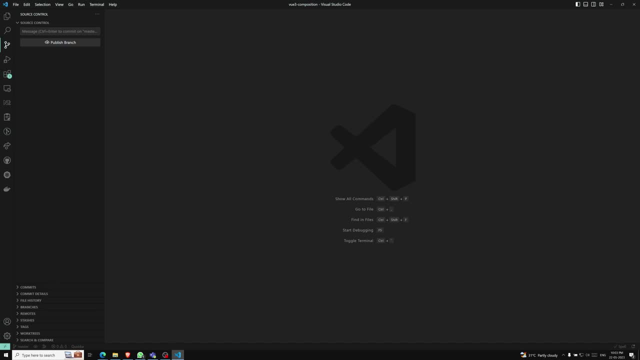 Those are nothing but vi-model, vi-show, vi-if. like this, we have the set of directives right. So like this: these are normal directives, So default directives. In addition to that, Vue also allows us to register your own custom directives also. We already introduced two. 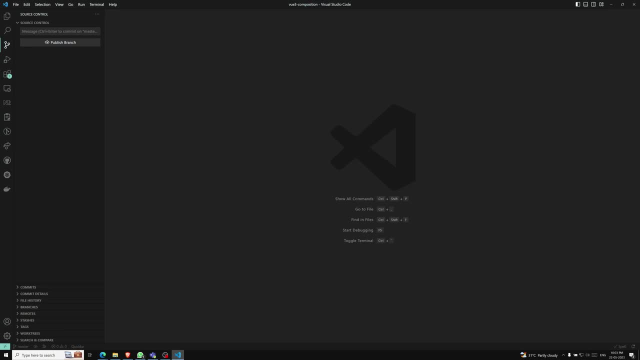 forms of code reuse, that is, components and also the composables. So these are the two things which we can make the code reusable. Components are the main building blocks, while composables are focused on reusing the stateful logic. So where this custom directives act? 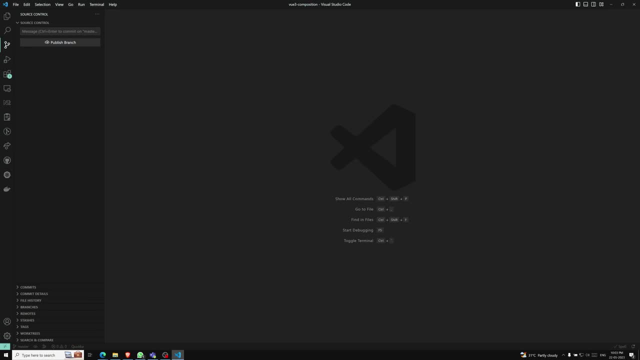 actually fit in. Custom directives, on the other hand, are mainly intended for reusing the logic that involves low level DOM access on the plain elements. That is the main thing. The custom directive is defined as an object. It is defined as a plain object containing 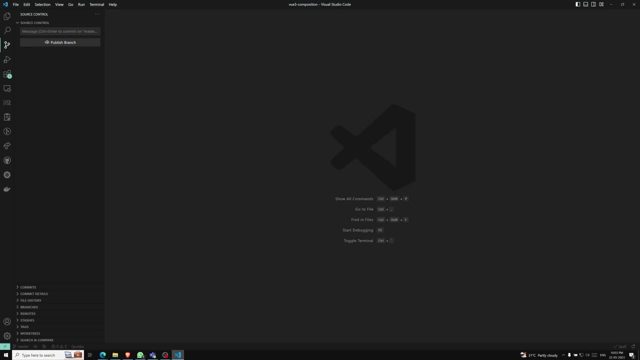 the lifecycle hooks similar to those of a component. These hooks receive the element the directive is bound to, And also we have other things like argument bindings and all those things we'll be having. I will try to show you a simple basic example How this custom directive will be. Let's say we have a single post, We already have this. 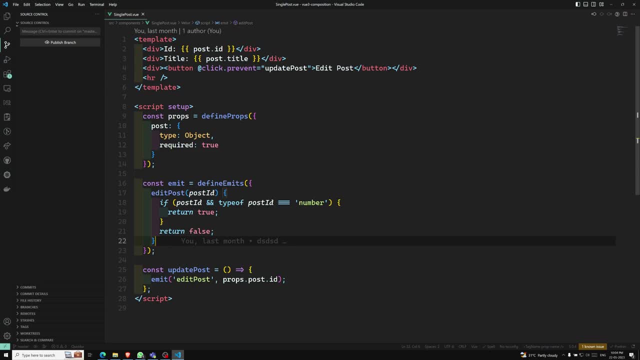 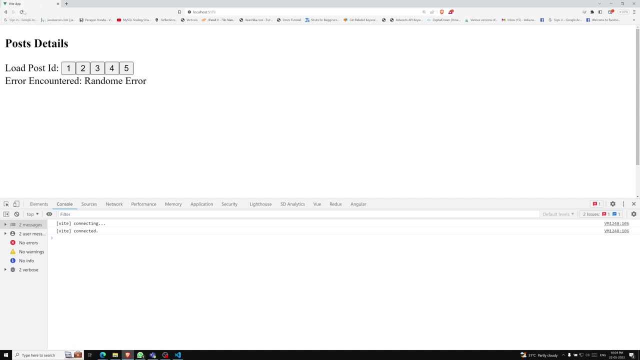 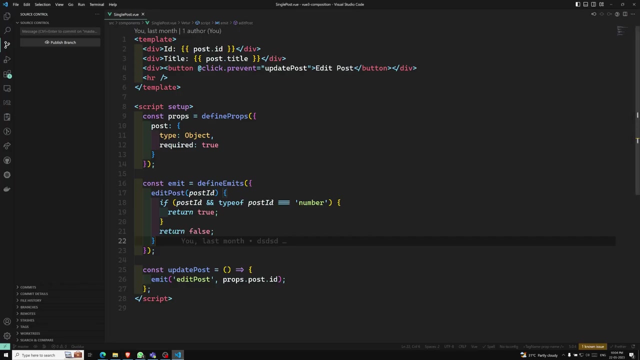 single post. right, This is our single post. You see the output here. You see the output in this one. This is our output In this output, which here we are having edit post. Now what I want to do is, let's say, we have an input box. Here I am having an input box. Type is: 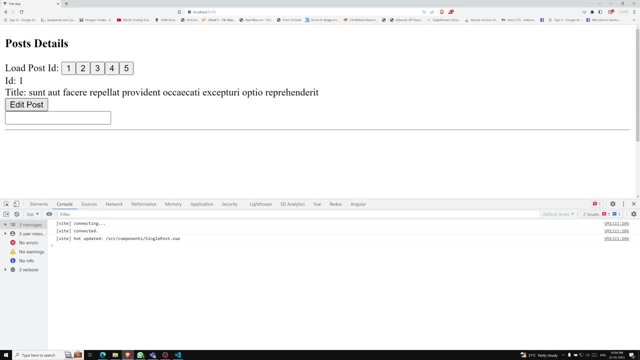 equal to text. Normally we are having this one. If you see, here we are having an input box. Now what I want to do is, whenever I am trying to do this one, automatically, this one has to autofocus. So this is the thing I wanted. So what can I do is we can create our custom. 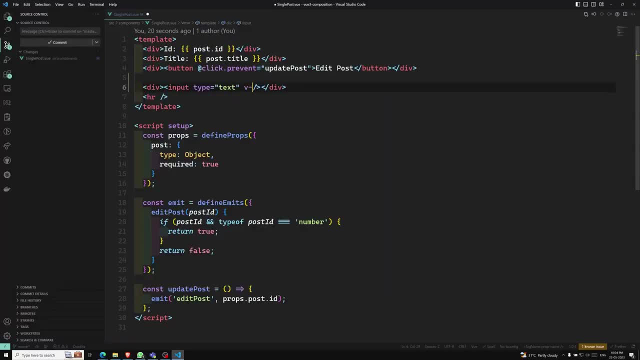 directive. How can I create our custom directives Here? I can use v-focus, So which is our custom directive? I am using v-focus And now how we can define this one in the composition, API is constant. v-focus is equal to. I told you, right Directive is a simple. 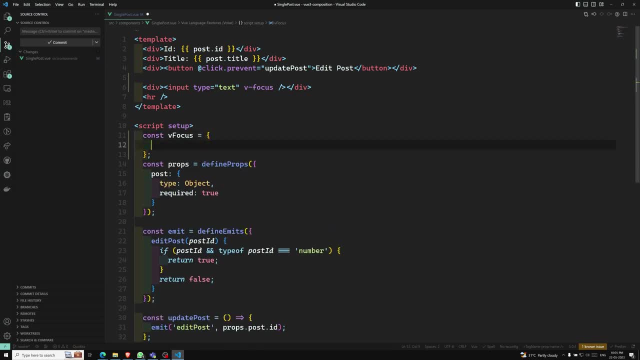 object. So, like this, we need to create an object And in this object we will be having the lifecycle hooks or anything, So I can create with a mounted. So this has an argument element. So this gives the element that is bound to. So here this element is bound to. 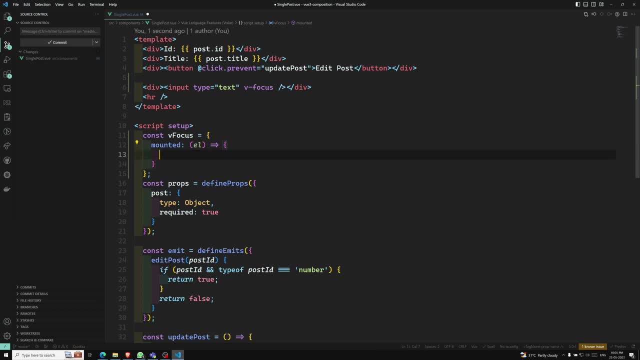 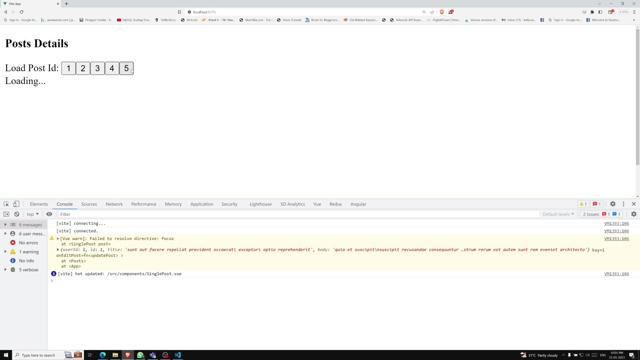 the input element, And here element is nothing but an input element. And now if I want to do el dot focus, That's it Now. automatically this will be focused. We try to see here output, See here, Automatically it will be focused. If you go here into the three, four, five, Yeah, Here it will be focused. 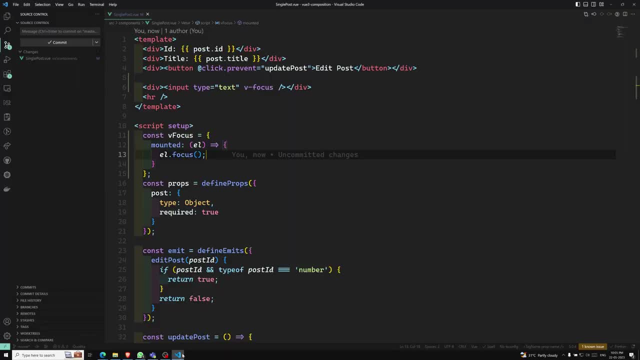 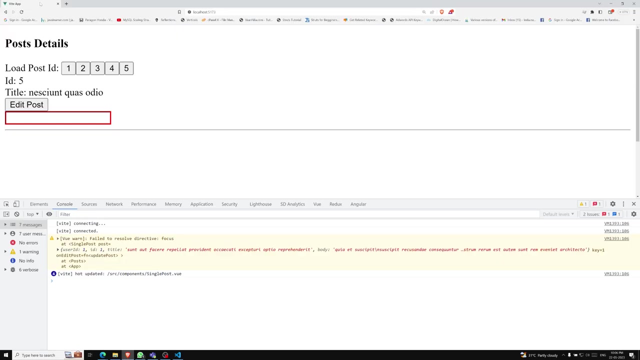 If you want to show something like what I can say- Background color, if you want to change it, So border color Also, you can change it to right. That's it. You see the output here. So this is how we can create a custom data, The basic custom data, how we can create it. 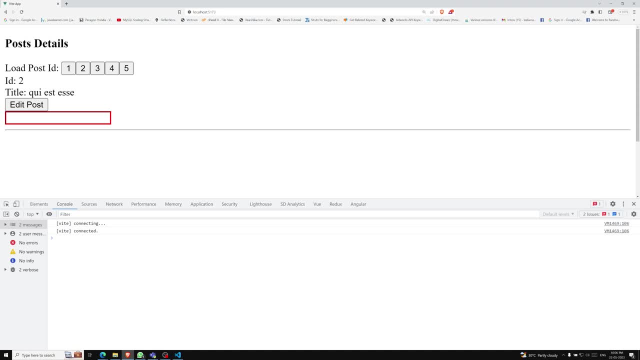 Normally what the director is, so the director which we have created, So this one will auto focus the input element. This director is more useful than the auto focus attribute, So normally we have an auto focus attribute, We can have this director. So using like this: 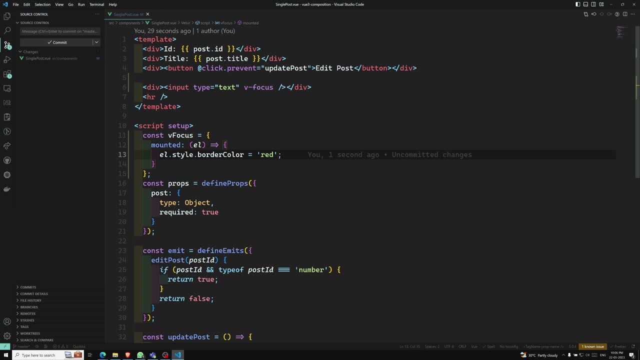 auto focus using the directories more useful because it works not only just on the page Load, it also works when the element is dynamically inserted by the view. So when the element is dynamically inserted by the view, then also this auto focus works, for which you have. 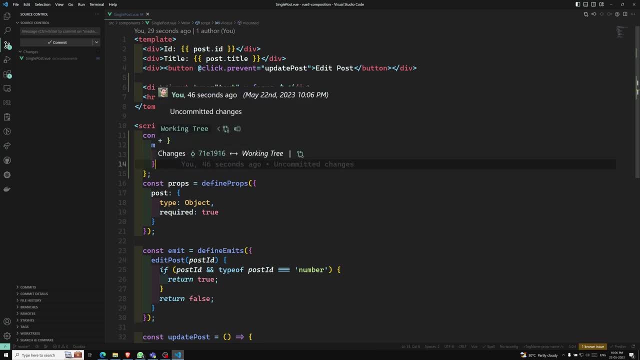 used it with the director. So that is the main thing in script setup. Any camel case variable that starts with the V prefix can be used as a custom directive. In the example above which we are trying to see, we focus can be used in the template as V, if and focus. 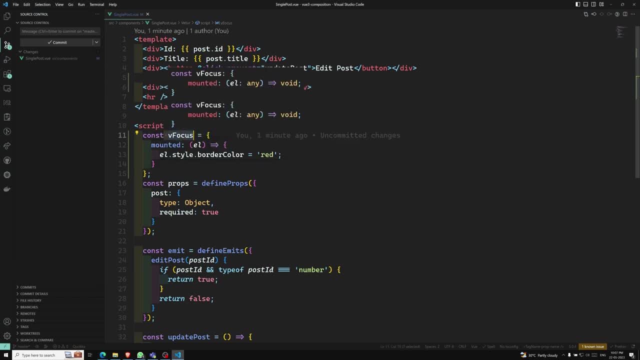 So here we are having as a prefix V right. So this is can be used as a custom directive and in this one. So here we can use it in the template as V, if and focus. So this is one thing which I want to tell you, If you. 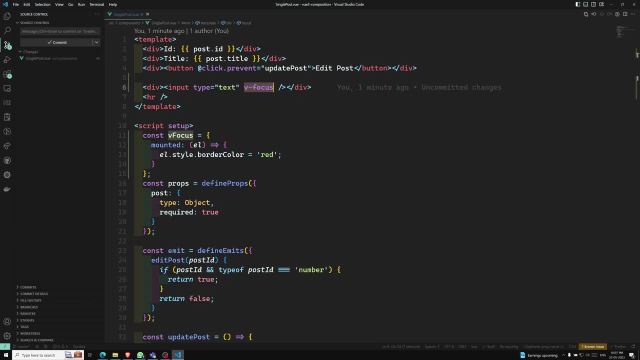 are not using the script setup means then you can have a directives option and you can use it. So not only like this, we can also create the custom direct to globally so that this custom data which we have created now it is only registered locally. So that means 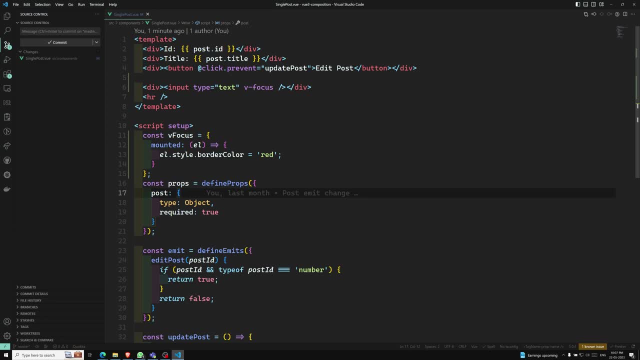 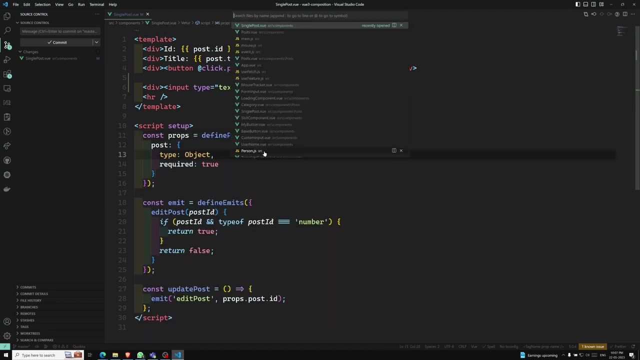 it will be registered only to this component. So if you want to make this direct to available to globally, So if you want to make this direct to available to globally, then you can remove this one all and let's go to the main dot J S. So here you can register that direct to how we can. 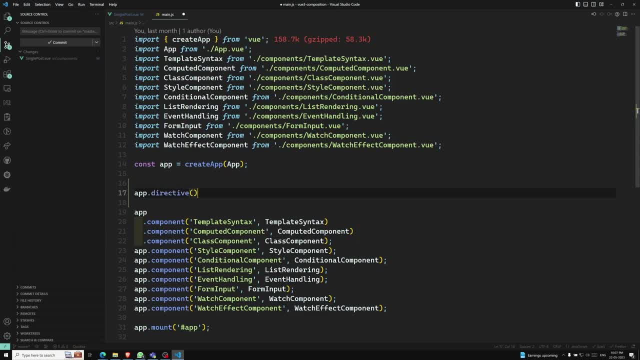 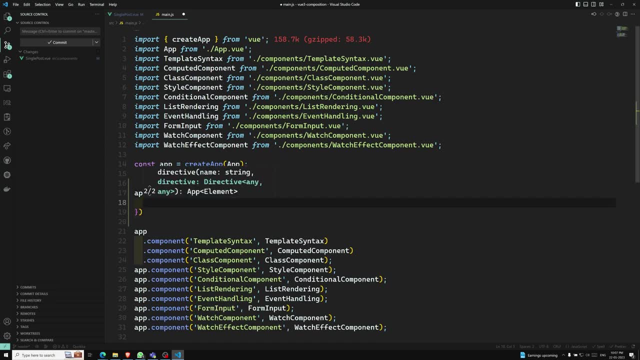 register. the direct is app dot direct to and the name of the direct to focus. So there is no need to mention the prefix and we will be having an object. in this one We will be having a mounted. We can also use it like this element. We got the element and in this, 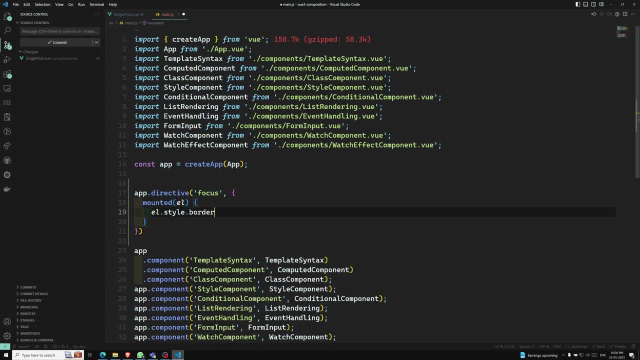 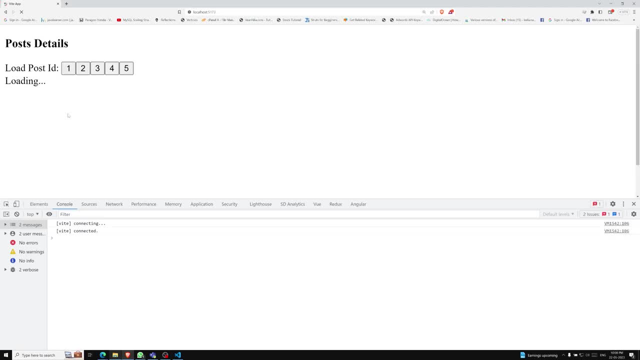 element. you can write: So: element dot, style dot, border color is equal to a low, will change it to a low so that we can be able to see the output. Now, if you see the output here, I click on the second, one, third one. Yeah, here we are able to see this in a local. So now the custom direct. 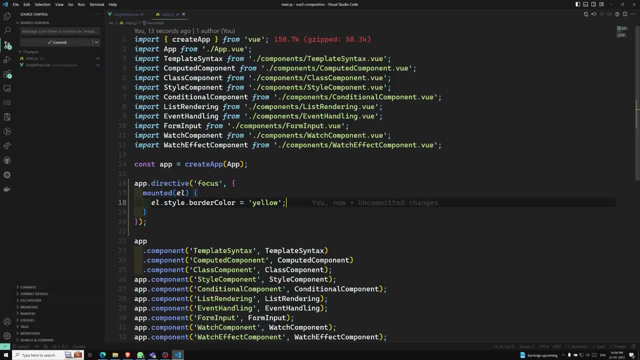 to which we have created globally. this can be used in any component. So this is one thing, so we can create the custom direct to both in the component level and also we can also register the custom direct to in the app level. So that is the main thing. Custom direct to should only be used when the desired functionality. 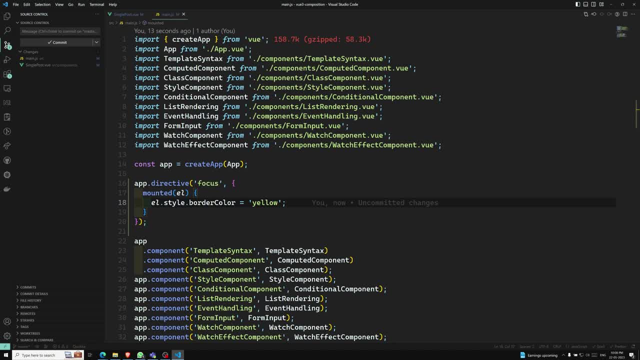 can only be achieved by a direct dom manipulation. preferred declarative templating using built in direct to, such as vif and bind, and possible because they are more efficient and server rendering friendly. So that is the main thing. So, whenever you prefer dom manipulation direct, 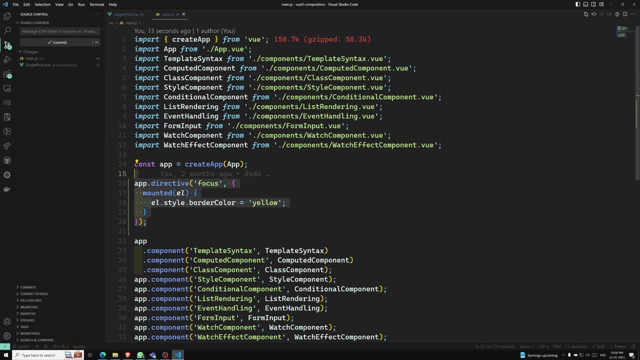 dom manipulation means it is preferable to use the custom direct to, most of the time, try to use the built in direct to solve it. So that is one thing. Now we have understood about the basic creation of the directives, So how the directives can be created and how. 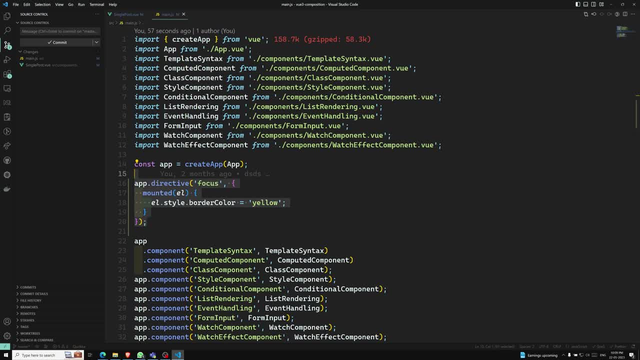 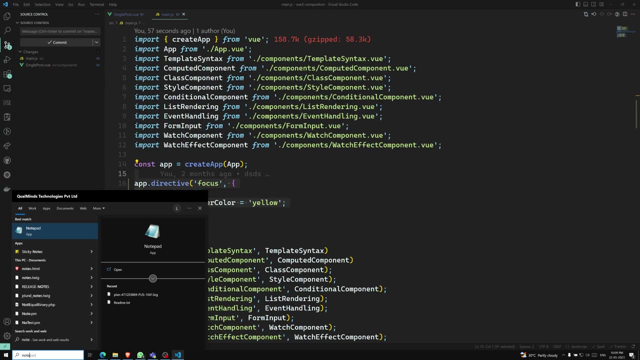 the directives is useful to us. So we have seen the basic thing. And the next one which I want to tell you is the direct to hooks. Okay, So, this is also one of the important concept. So, direct to in the direct to books, I want to show you to open this, Okay so,